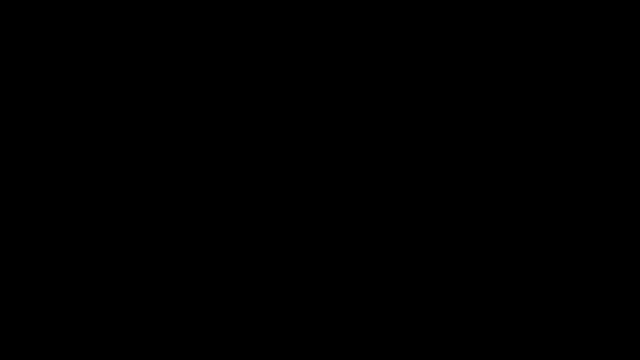 In this video we're going to focus on finding the missing side of a triangle. if we're given two similar triangles, So let's start with an example. So let's say that these two triangles are similar to each other: The triangle on the. 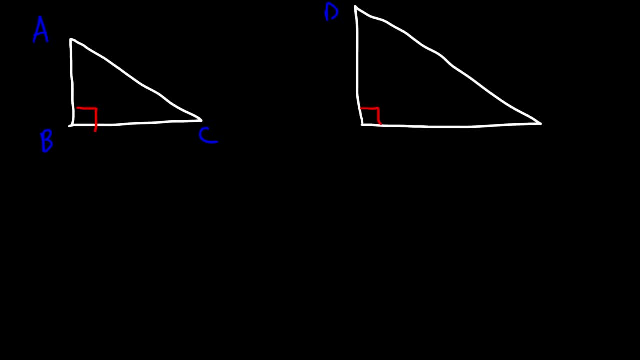 left. let's call it triangle ABC and this is going to be triangle DEF, And let's say that segment AB is 8 and BC is 6.. DE is 12 units long and our goal is to find the missing side EF. So we're going to place an X there. 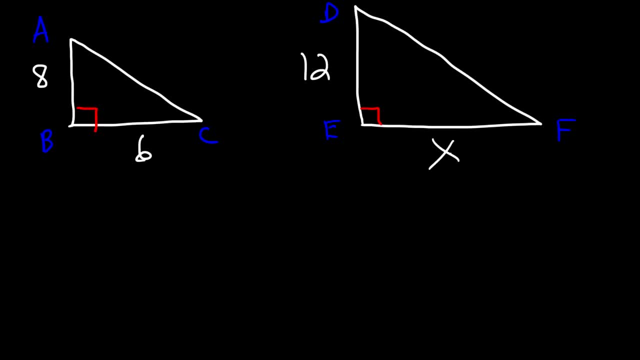 So how can we find the value of X? In addition, let's say that angle A is similar to angle D and angle C is congruent to angle F, Subsequent. So, with this information, what can we do to find the value of x? 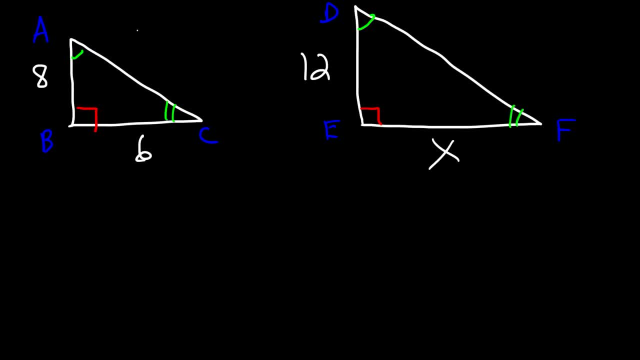 What we need to do is set up a proportion. Let's call this triangle T1 and this triangle T2.. So I'm going to have two fractions separated by an equal sign. On the left, I'm going to put the information associated with triangle 1.. 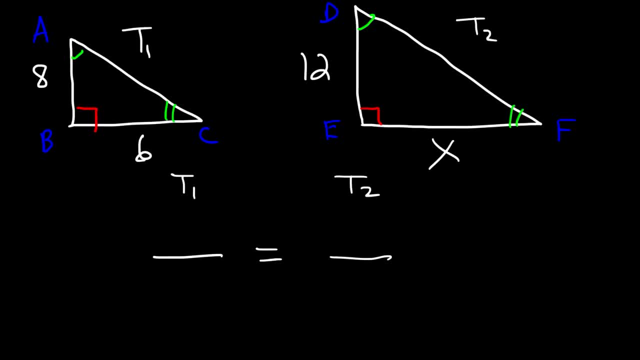 On the right triangle 2.. On the numerator of triangle 1,, that's going to be 8.. Now, 8 is similar to 12.. These two sides correspond to each other. This one- 6, is going to be the denominator for triangle 1, and that is similar to x for 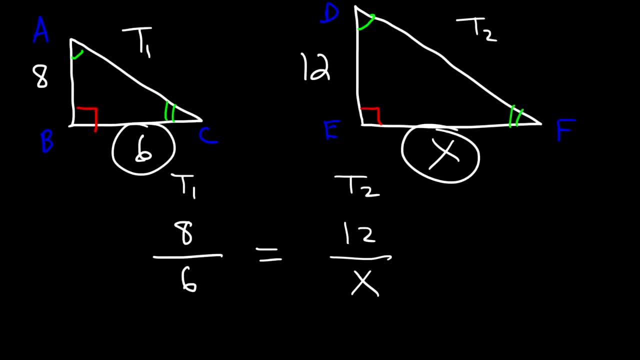 triangle 2.. So that's how you can set up the proportion. Now, in order to solve it, We need to cross multiply. So 8 times x, that's 8x, and that's going to be equal to 6 times 12, which is 72.. 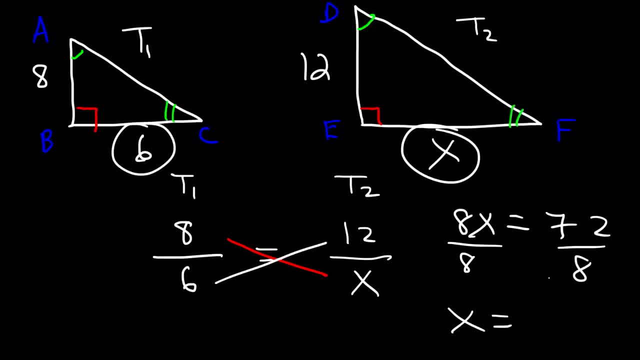 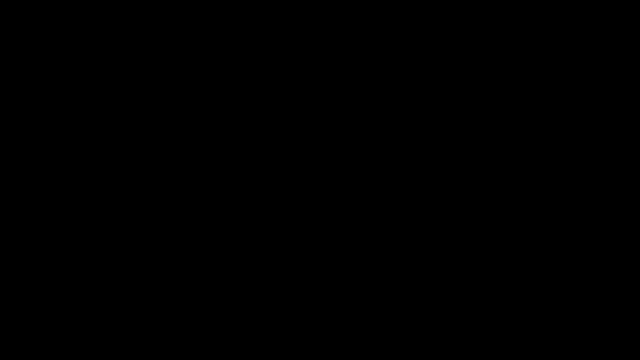 So now all we need to do is divide both sides by 8, 72 divided by 8 is 9.. So that's going to be the answer: x is equal to 9.. Now let's work on another example. Okay, 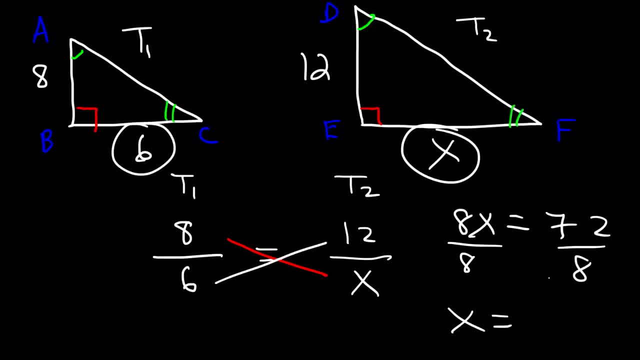 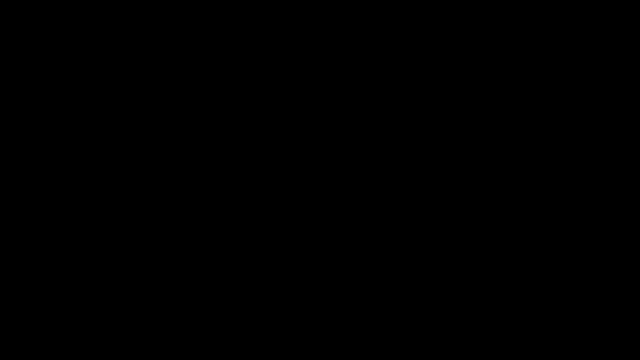 So now all we need to do is divide both sides by 8, 72 divided by 8 is 9.. So that's going to be the answer: x is equal to 9.. Now let's work on another example. Okay, 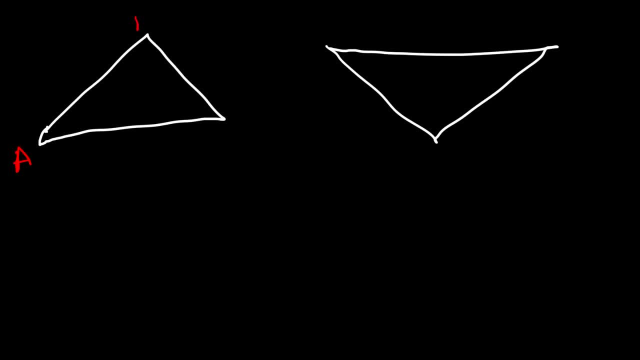 So let's say this is triangle ABC and this is DEF. Let's say that AB is 18 and BC is 24.. And let's say that angle A corresponds to angle F, Angle B corresponds to angle F, Angle B corresponds to angle F. 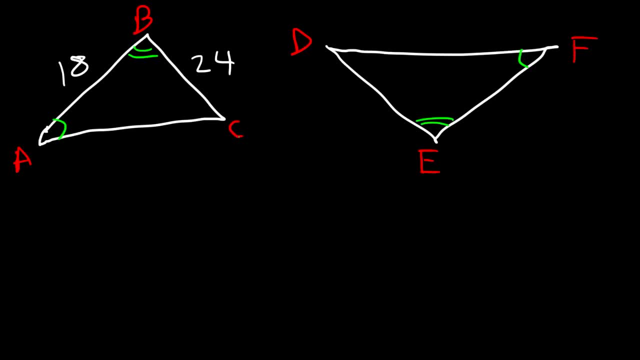 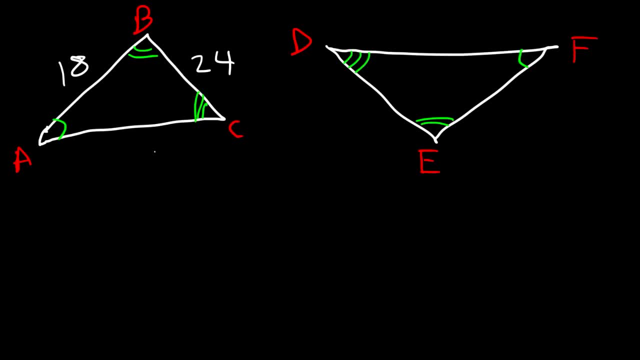 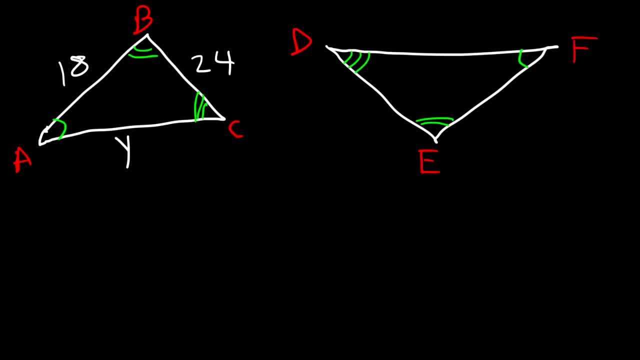 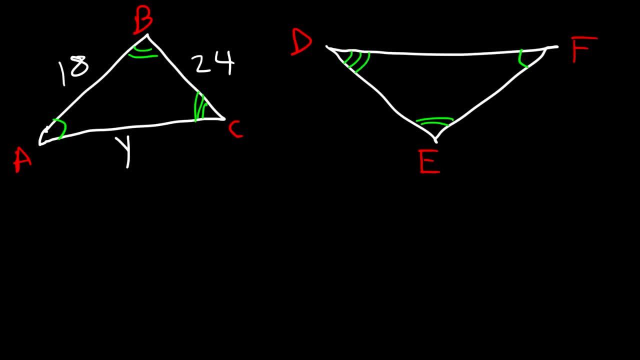 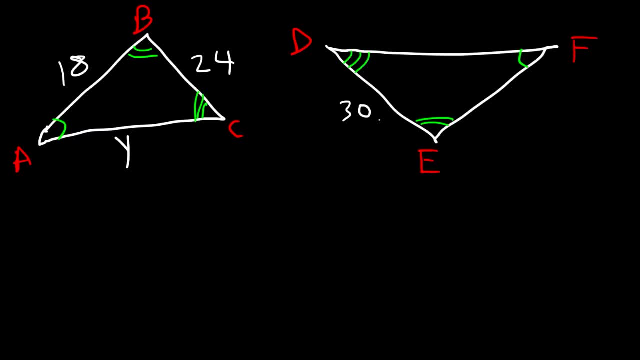 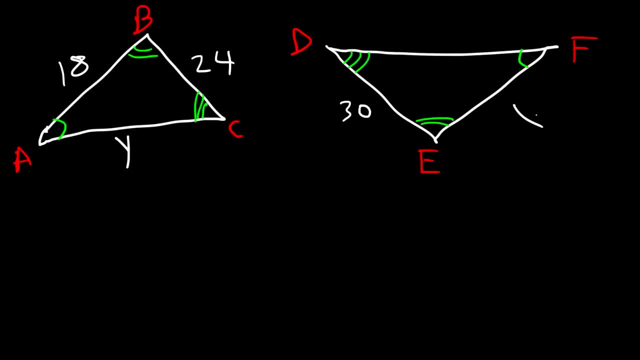 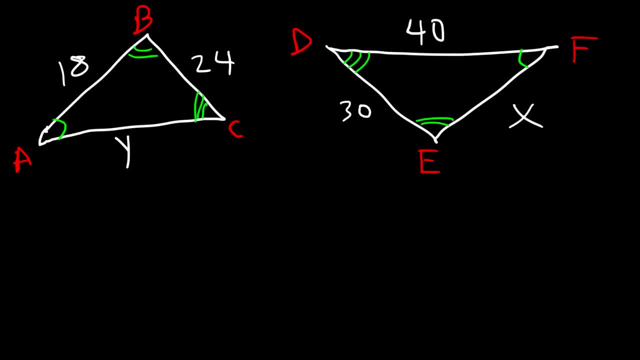 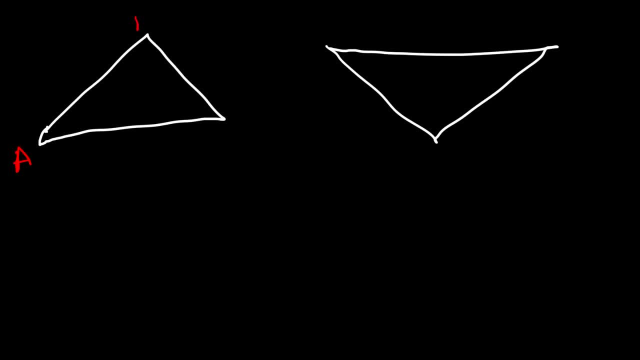 So let's say this is triangle ABC and this is DEF. Let's say that AB is 18 and BC is 24.. And let's say that angle A corresponds to angle F, Angle B corresponds to angle F, Angle B corresponds to angle F. 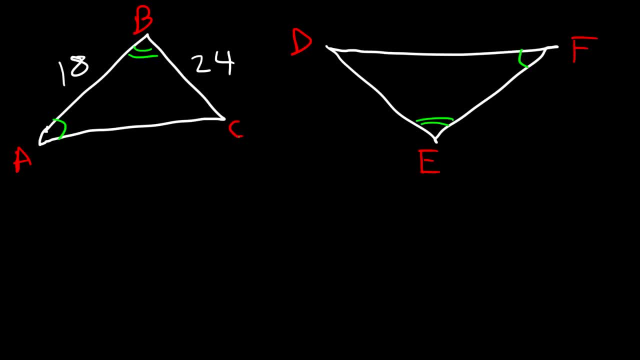 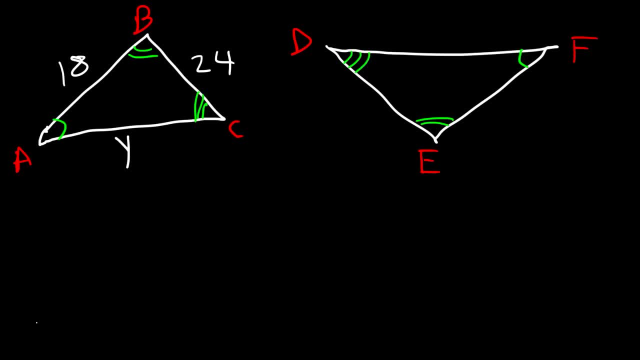 Actually not 16.. 1.. 1?, 1?? And let's say that EF is X and let's make DF 40. Go ahead and find the values of X and Y in this problem. So let's start with X. 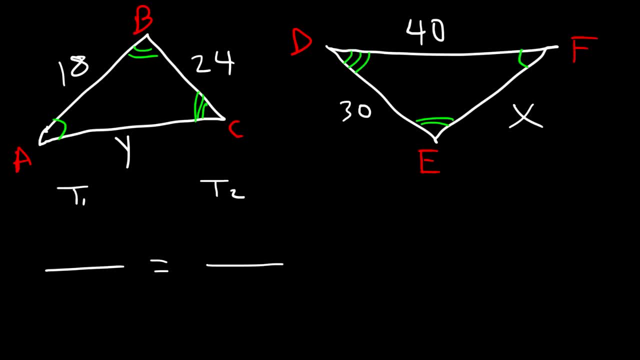 This is going to be for triangle 1 and triangle 2.. Now we're going to say triangle 1 is the one on the left, Angle A, which is associated with 24, that corresponds to angle F. So if we put 24 on, 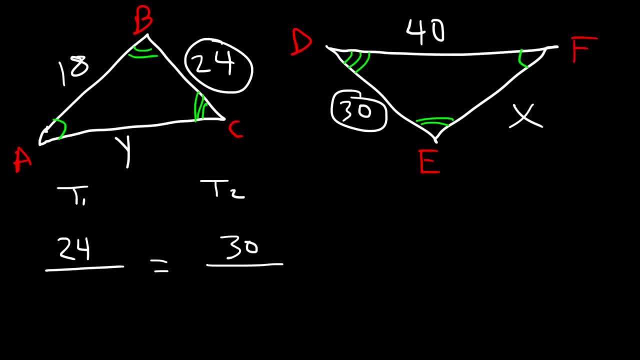 top of triangle 1, we need to put 30 on top of triangle 2.. Those two sides correspond to each other Now 18. 18.. 18,, which is associated with angle C. it's opposite to, it is similar to angle D, which 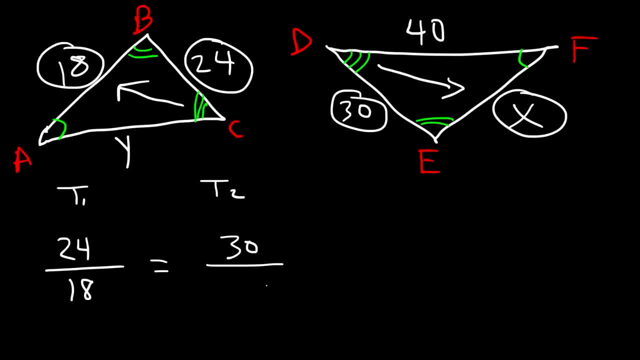 is associated with X, So we're going to put 18 and X. So now let's cross multiply, So first we have 18 times 30, and that's equal to 24 times X. Now, to make the math easier, you can break down the numbers into smaller numbers. 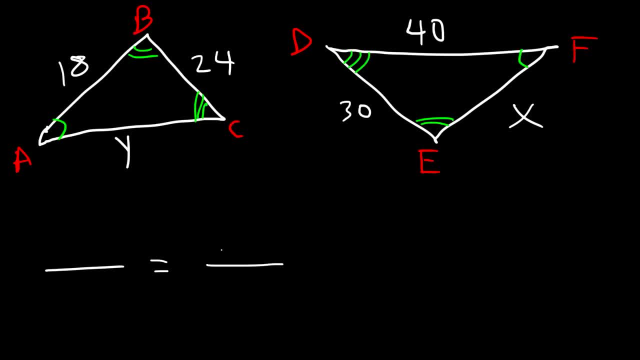 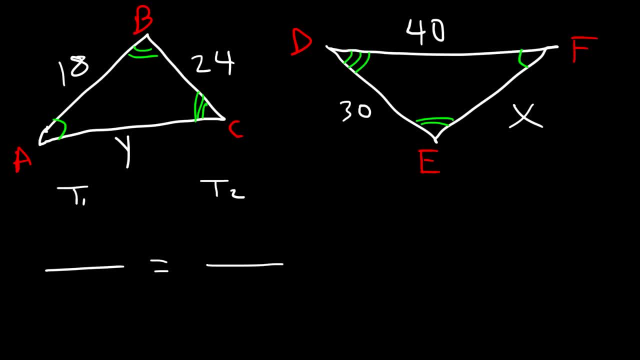 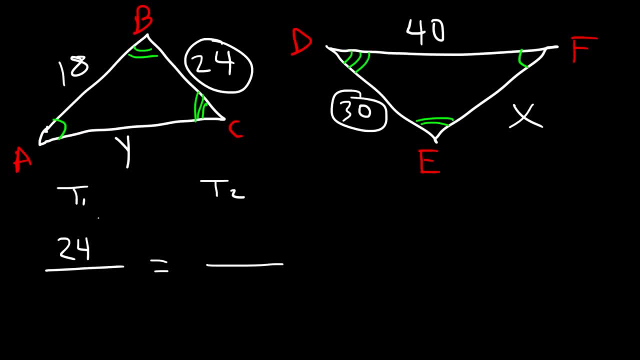 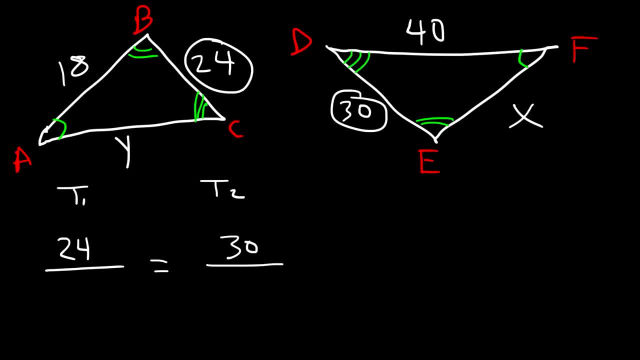 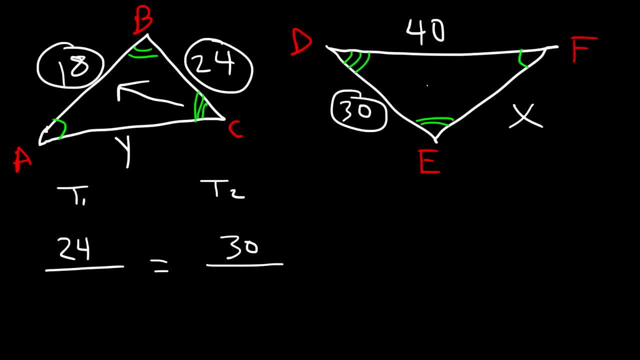 Angle B corresponds to angle F. angle C, it's opposite to it, is similar to angle D, which is associated with X. So we're going to put 18 and X. So now let's cross multiply. So first we have 18 times 30, and that's equal to 24 times X. 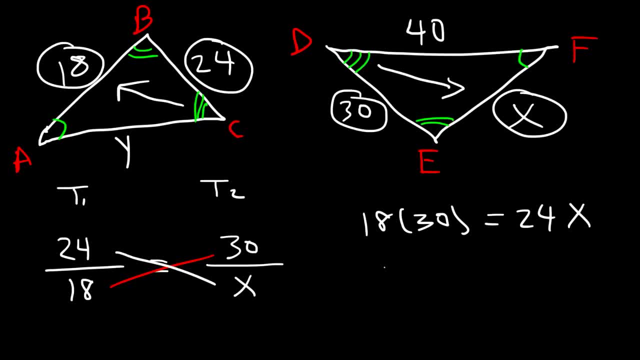 Now, to make the math easier, you can break down the numbers into small numbers. For example, 30 is 6 times 5, and 18 is 9 times 2.. 24 is 6 times 4, and 4 is 2 times 2.. 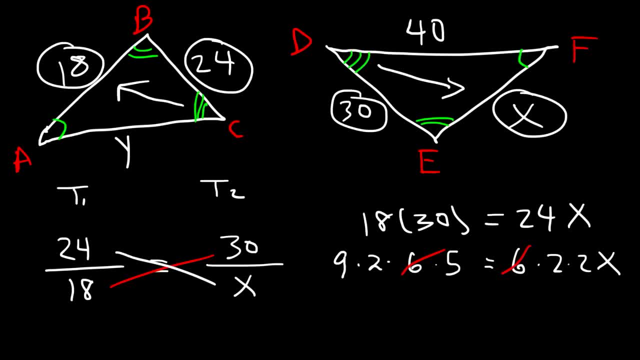 So notice that you can cancel a 6, and you can cancel a 2,, which will make life easier. 9 times 5 is 45,, so 45 is equal to 2X, And if you divide both sides by 2,, X is 2.. 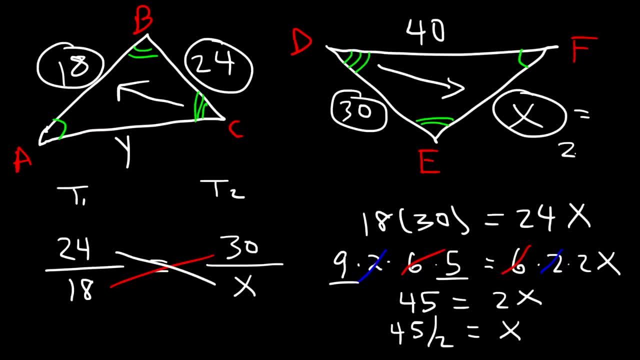 That's 45 over 2, which as a decimal is 22.5.. So that's the value of X. Now let's find the value of Y. Let's set up another proportion between triangles 1 and 2.. So, just like in the last example, we know that angle A is still congruent to angle F. 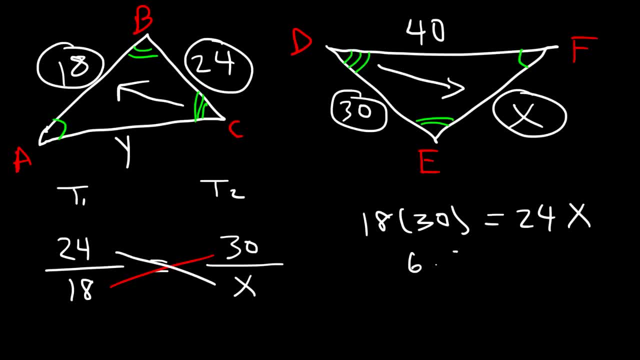 For example, 30 is 6 times 5, and 18 is 9 times 2.. 24 is 6 times 4, and 4 is 2 times 2.. So notice that you can cancel a 6, and you can cancel a 2,, which will make life easier. 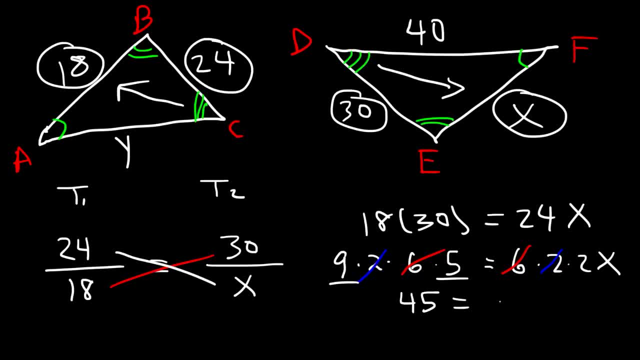 9 times 5 is 45, so 45 is equal to 2X, and if you divide both sides by 2, X is 45 over 2.. So that's the value of X. Now let's find the value of Y. 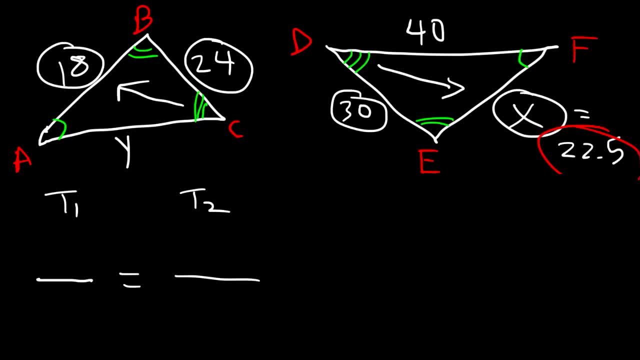 Let's set up another proportion between triangles 1 and 2.. So, just like in the last example, we know that angle A is still congruent to angle F, So 24 corresponds to 30. So we can put that on top again. 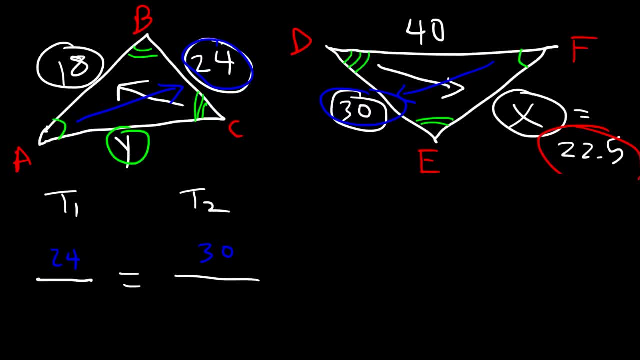 Now, angle Y- I mean not angle Y, but side Y- has to correspond to 40. Angle B and angle E are congruent to each other, So Y and 40, they're on similar sides. So now that we have the proportion, we can go ahead and solve it. 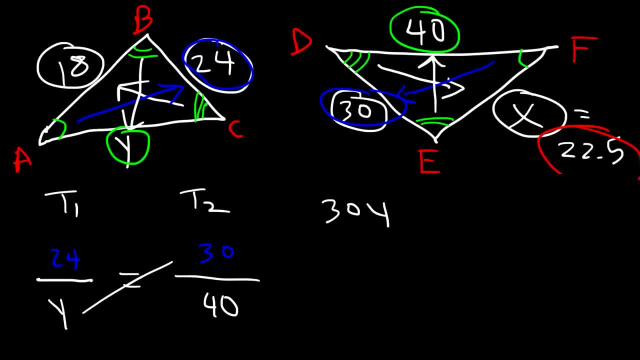 So let's cross multiply. We're going to have: 30 times Y is equal to 24 times 40. So let's see if we can simplify our answer without the use of a calculator. 30 is 3 times 10.. 24 is 3 times 8, and 40 is 4 times 10.. 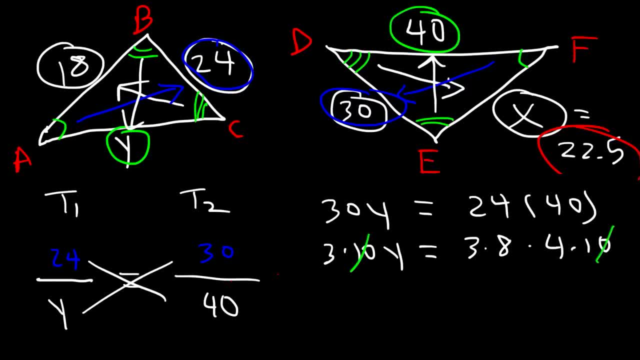 So we can cancel a 10 from both sides and we can cancel a 3.. So what we have left over is Y times Y. Y is equal to 8 times 4, and 8 times 4 is 32.. So that's the value of Y in this problem. 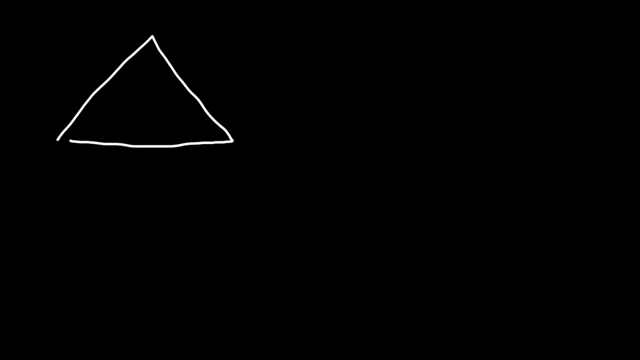 Here's another example that you could work on for the sake of practice. So, once again, this is going to be triangle ABC and this is triangle DEF. Let's say that this is 15.. And this is 15.. And this is 15.. 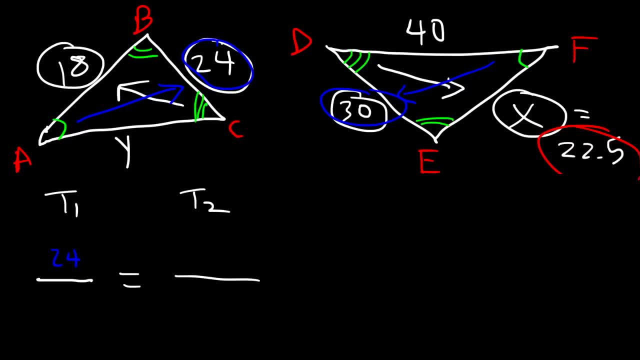 So 24.5.. Corresponds to 30. So we can put that on top again Now. angle Y- I mean not angle Y, but side Y- has to correspond to 40.. Angle B and angle E are congruent to each other. 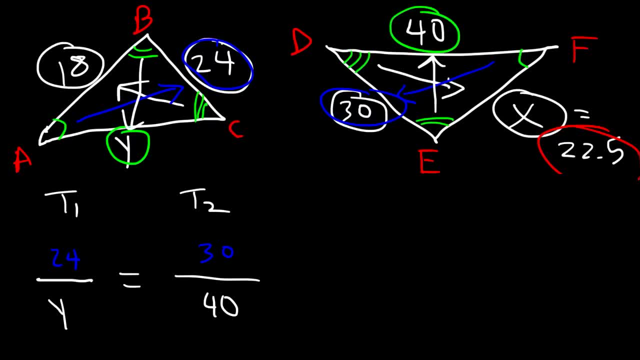 So Y and 40, they're on similar sides. So now that we have the proportion, We can go ahead and solve it. So let's cross, multiply. We're going to have 30 times Y is equal to 24 times 40.. 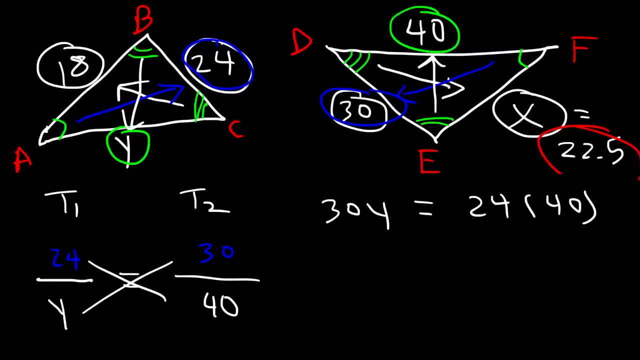 So let's see if we can simplify our answer without the use of a calculator. 30 is 3 times 10.. 24 is 3 times 8. And 40 is 4 times 10.. So we can cancel a 10 from both sides. 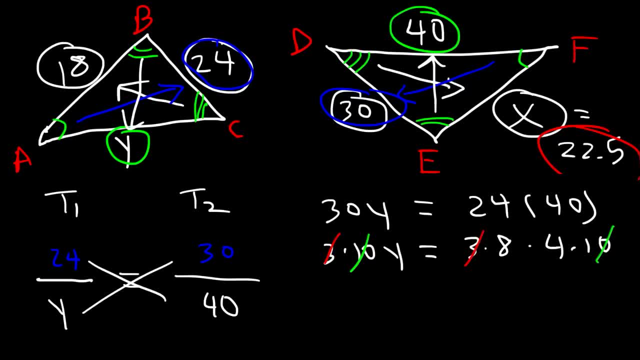 And we can cancel a 3.. So we can cancel a 3.. So what we have left over is Y is equal to 8 times 4. And 8 times 4 is 32.. So that's the value of Y in this problem. 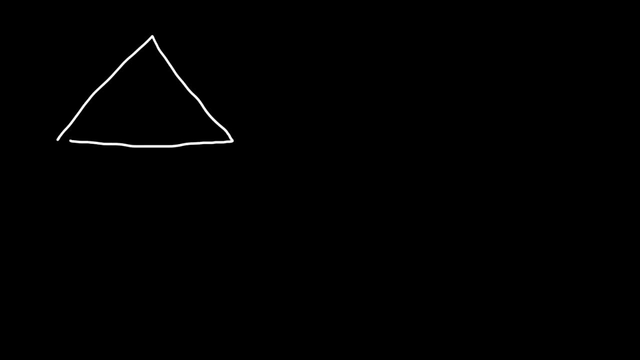 Here's another example that you can work on for the sake of practice. So, once again, this is going to be triangle ABC And this is triangle DEF, Okay, So Okay, Let's say that this is 15 and this is 9.. 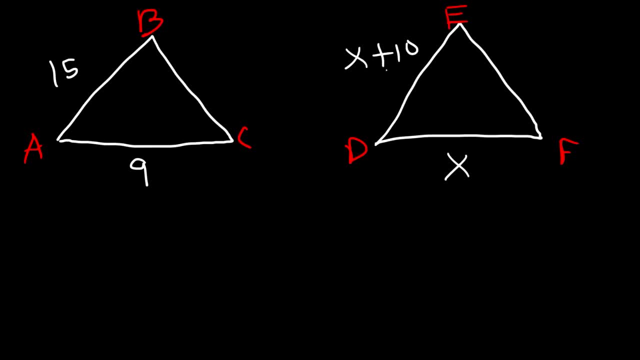 And this is X, And this side is X plus 10.. And let's say that angle A corresponds to angle D, Angle C corresponds to angle F And angle B corresponds to angle E. So, with this information, go ahead and find the value. 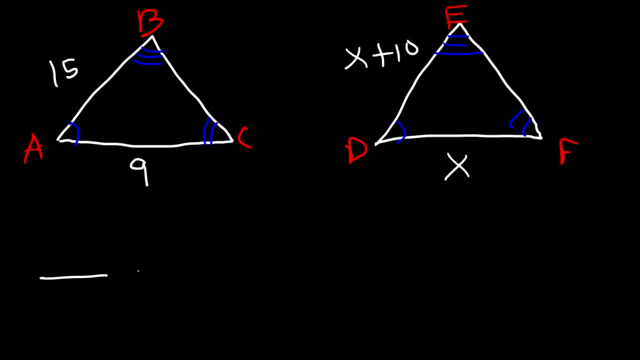 of X. Okay, So, just like before, let's create a proportion: 15 corresponds to X plus 10.. Because they're across two angles that are congruent- Angle C is congruent to angle F. Now 9 corresponds to X. 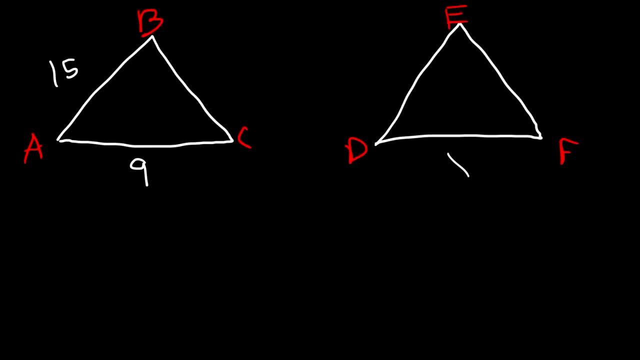 And this is 15.. And this is 9.. And this is 9.. And this is X, And this side is X plus 10.. And let's say that angle A corresponds to angle D, Angle C corresponds to angle F. 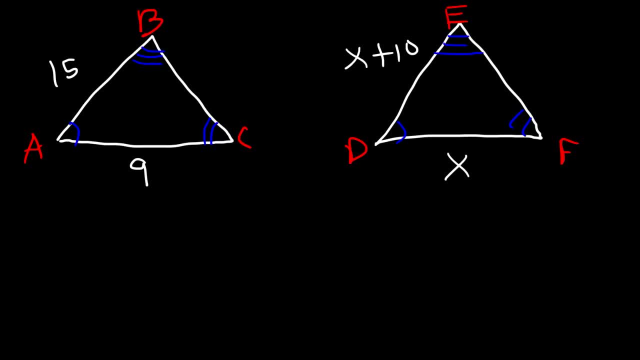 And angle B corresponds to angle E. So, with this information, go ahead and find the value of X. So, just like before, let's create a proportion: 15 corresponds to X plus 10, because they're across two angles that are congruent. 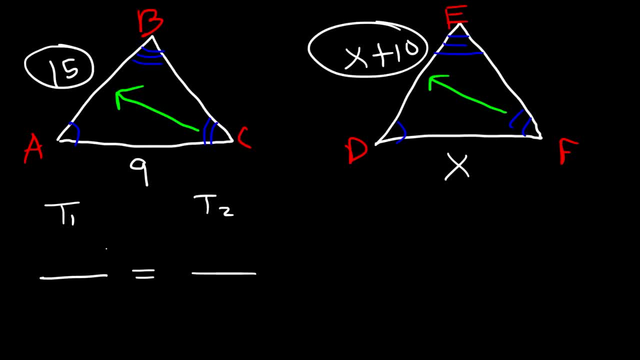 Angle C is congruent to angle F. Now 9 corresponds to X, because angle B and angle E are congruent to each other. So now we're going to find the value of X plus 10.. And now we're going to find the value of X plus 10.. 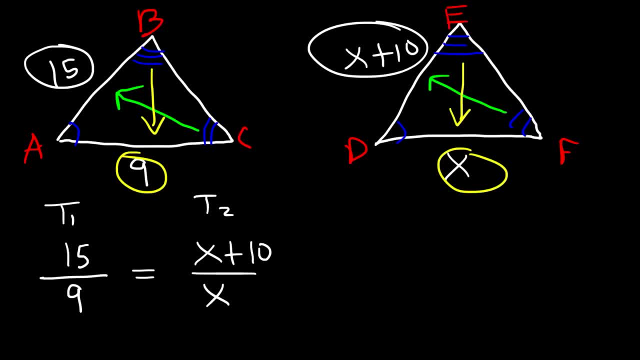 Angle X is congruent to X plus 10.. So now that we have this proportion, we can go ahead and find the value of X. So let's cross, multiply 15 times X is 15X, 9 times X plus 10.. 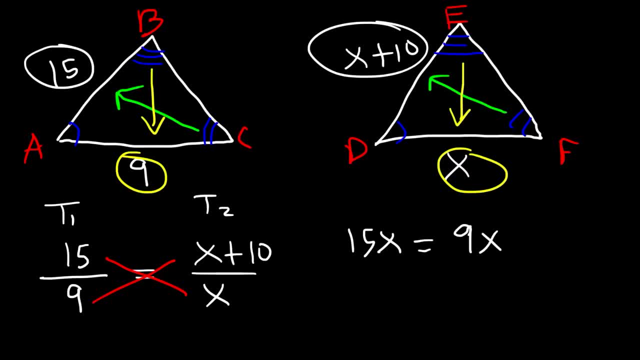 We need to use the distributive property, So that's going to be 9X plus 90.. 9 times 10 is 90.. So now let's subtract both sides by 9X. 15x minus 9x is 6x, so 6x is equal to 90. 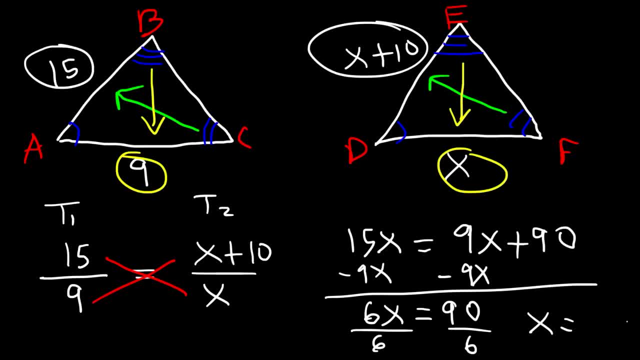 All we need to do is divide by 6,. 90 divided by 6 is 15,, so that's the value of x. So segment DF is 15 units long, DE is 15 plus 10, or 25.. So that's how you could find the two missing sides of this triangle. 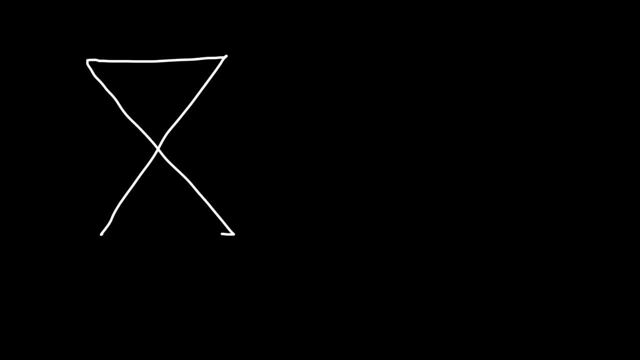 Let's try one last example. So let's call this angle: A, B, C, D and E. Let's say that AB is 8,, AC is 5,, BC is 7, DC is x, DE is 12.. 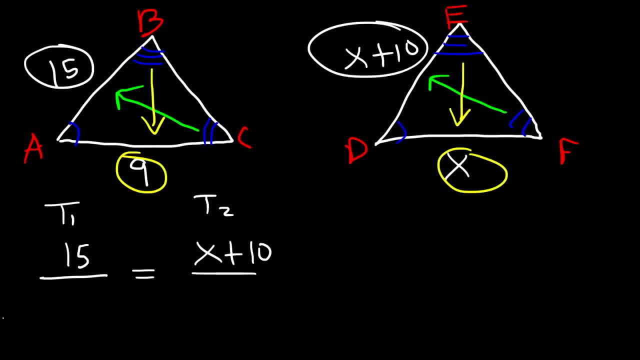 Because angle B and angle F are congruent, Okay Okay, And angle E are congruent to each other. So now that we have this proportion, we can go ahead and find the value of X. So let's cross, multiply 15 times. X is simply 15X. 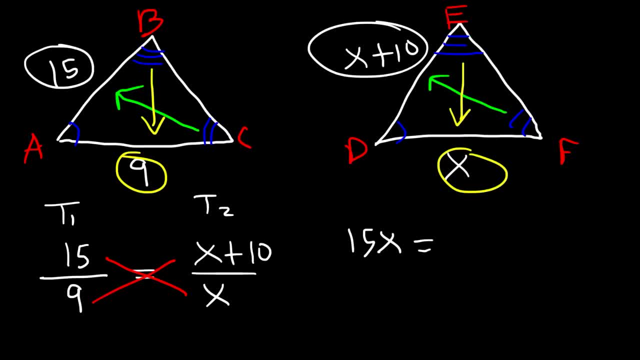 Nine times X plus 10.. We need to use the distributive property, So that's going to be 9X plus 90.. Nine times 10 is 90. So now let's subtract both sides by 9X, Okay. 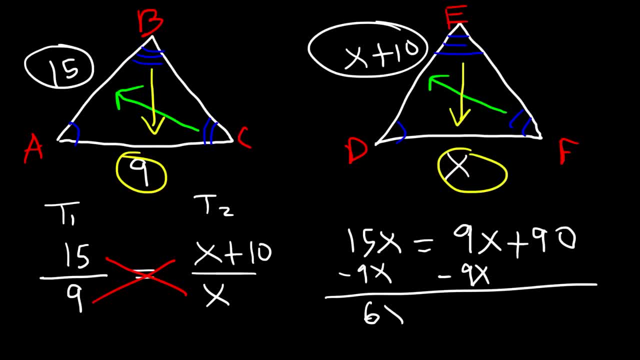 15X minus 9X is 6X, So 6X is equal to 90.. All we need to do is divide by 6.. 90 divided by 6 is 15.. So that's the value of X. 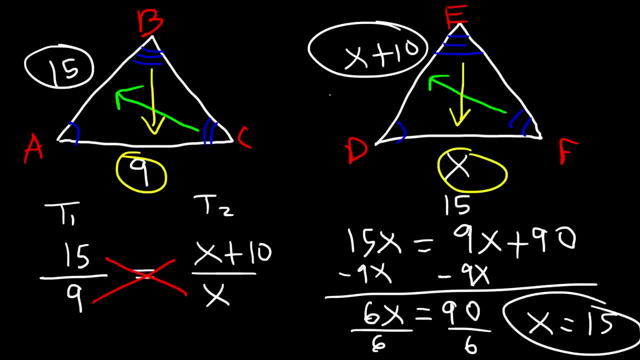 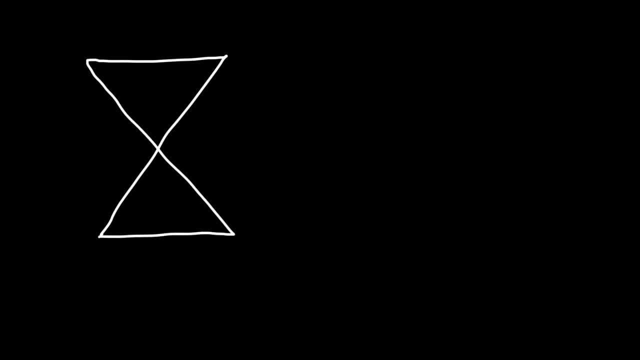 So segment DF is 15 units long, DE is 15 plus 10 or 25.. So that's how you could find the two missing sides of this triangle. Let's try one last example. So how many angles do we have? Let's say: 1., 2., 3., 4., 5., 6., 8., 9., 10., 11., 12., 13., 14., 15., 16., 15., 14.. 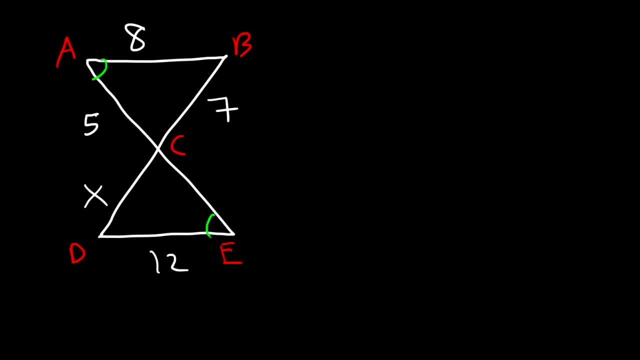 15., 25., 16., 17., 18., 21., 22., 23., 24., 25. 24. angle D Angle ACB is congruent to DCE. So with this information, go ahead and find X. 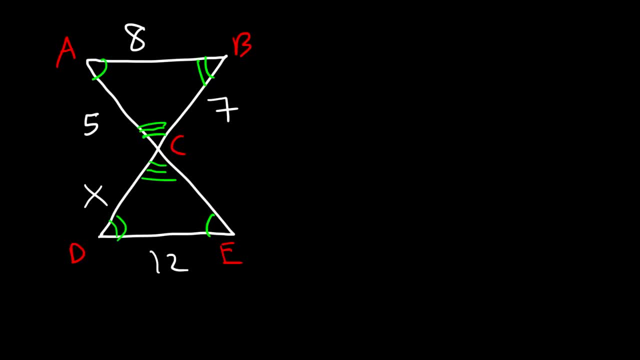 Let's call the top triangle triangle 1 and the bottom one triangle 2.. So let's set up a portion between T1 and T2.. Now, angle A is congruent to angle E, so that means 7 and X are similar to each other. Angle C: well, these two angles are equal to each other. 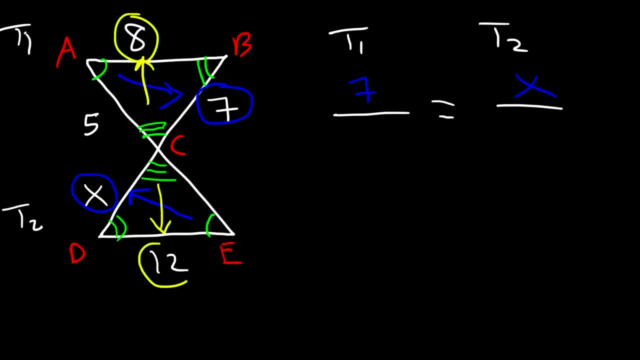 So 8 and and 12 correspond to each other. So now let's cross multiply: 8x is equal to 7 times 12,, 8 is 4 times 2,, 12 is 4 times 3, so we can cancel a 4..